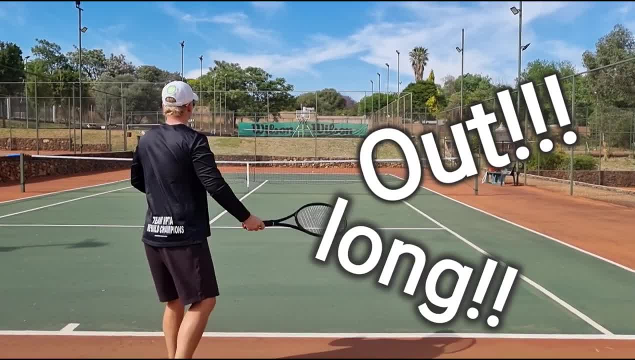 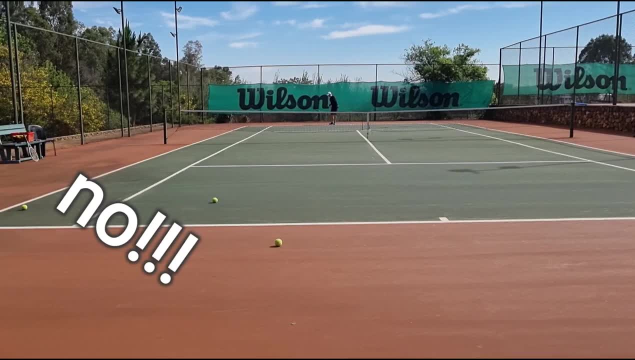 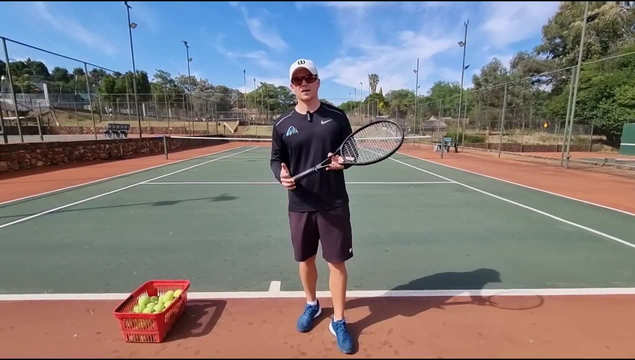 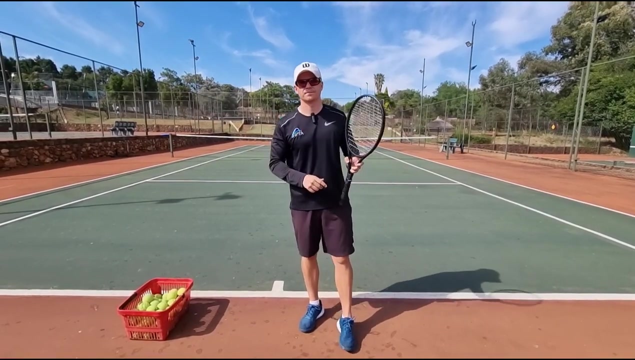 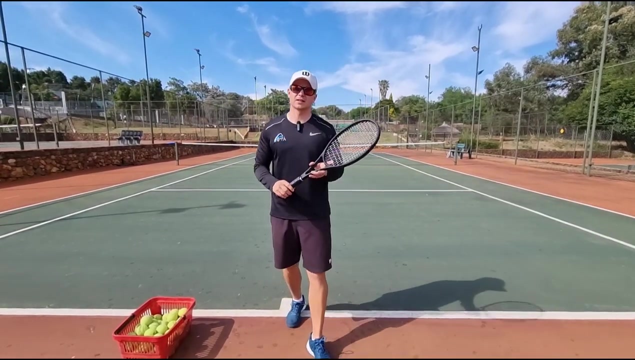 Are you always hitting the ball out and long, and you're just not sure why? Guys, I'm going to show you today three steps to help you to keep the ball in and to stop you from hitting the ball out all the time. Okay, guys, so the first very common mistake that players make and the reason why. 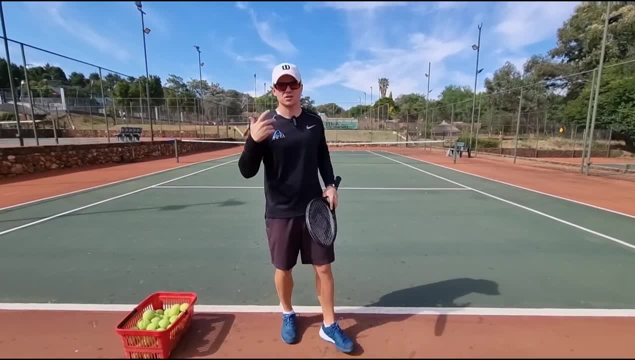 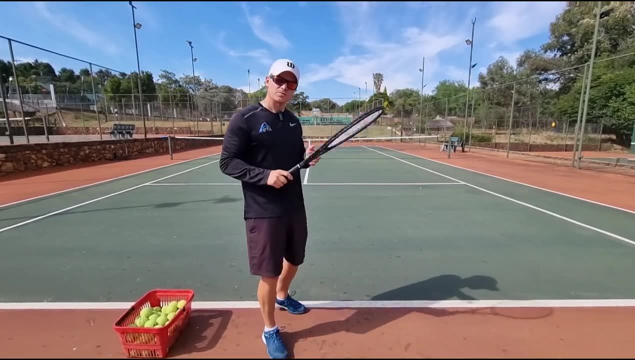 they're always hitting the ball out is. it sounds very basic, but it's so, so important. What's happening is you're not allowing your racket head to do the work, so what players do is- I've had the previous videos about this as well- is you're gripping the racket just too tight. so if 10 out, 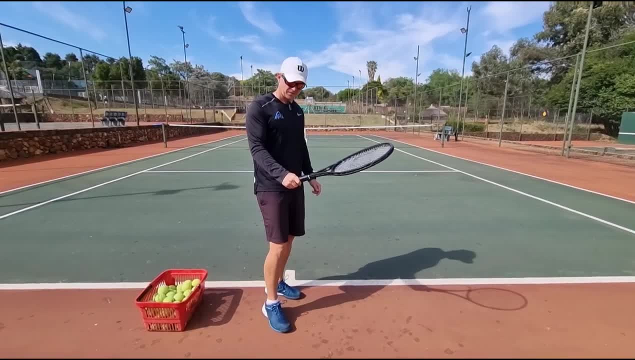 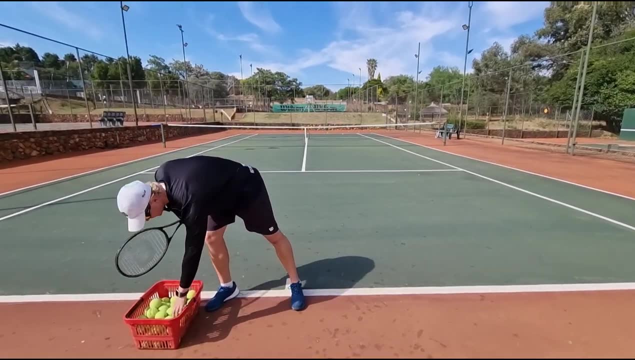 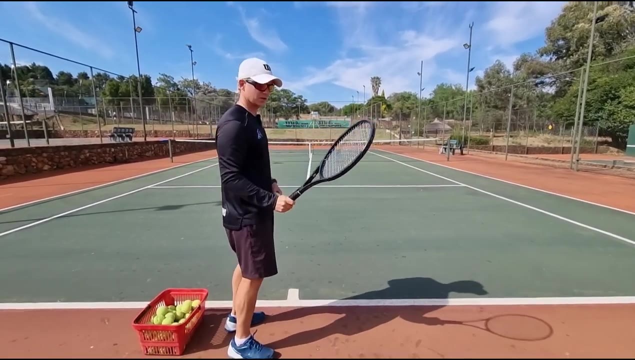 of 10 is as tight as you can. you want to be on around about 4 out of 10 so you can actually let the racket head do the work. because I'll show you an example: if you're gripping the racket too hard trying to get the ball in the court, it's very hard to get topspin, it's very hard to feel the ball. 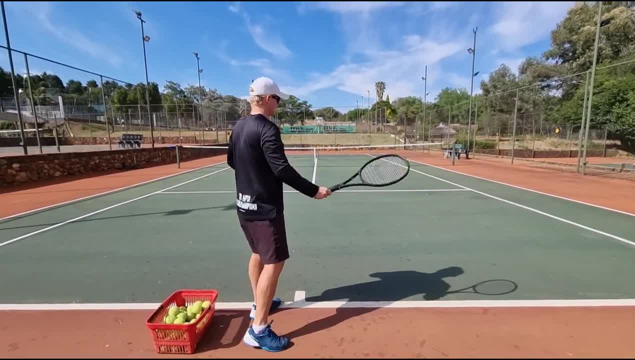 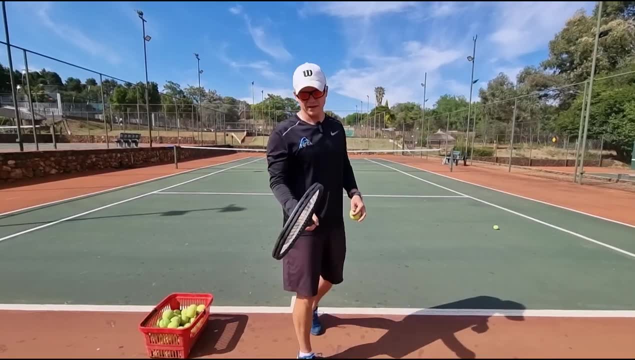 so the ball is just going to do its own thing. So it's so easy for that ball to go long and out when you're gripping it too hard. If it goes in, you're lucky, because you have no control In tennis. you've got to understand. 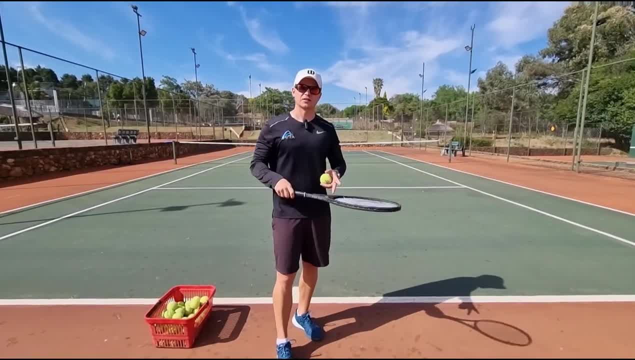 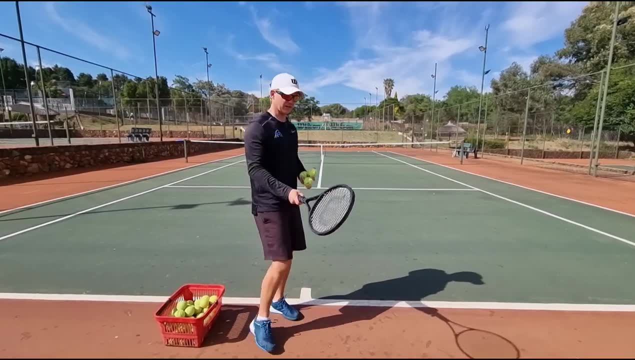 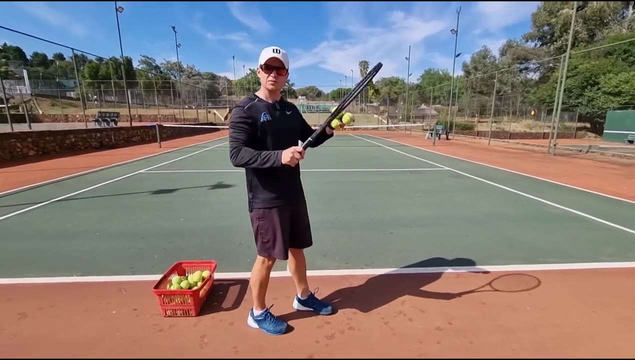 if you want more control, you almost have to let go of control. you know, let the control go into the racket. It's crazy as that sounds. so what I want you to imagine is relax, grip it 4 out of 10 and then notice now how my racket head is just going to go over the ball effortlessly and 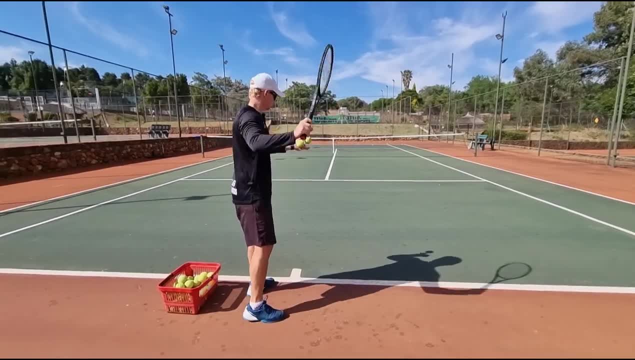 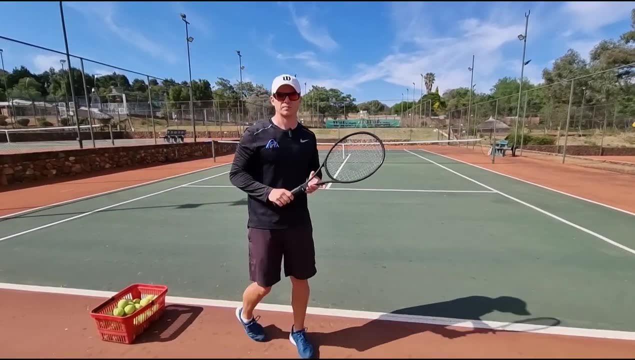 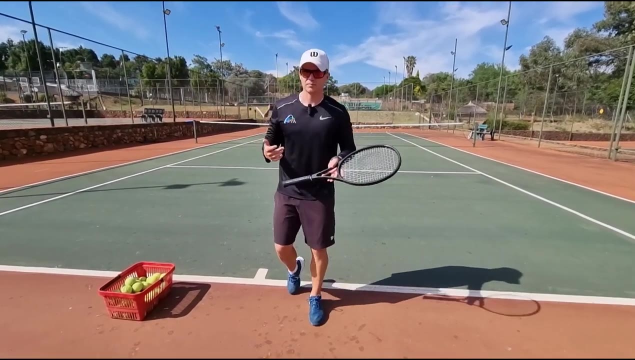 allow the ball to dip in. Just relax. notice how that ball you is dipping in. Try that the next time you play guys. Step number two: mistake number two that players make is again, it's going to sound common, but you've got to understand that if you open up, 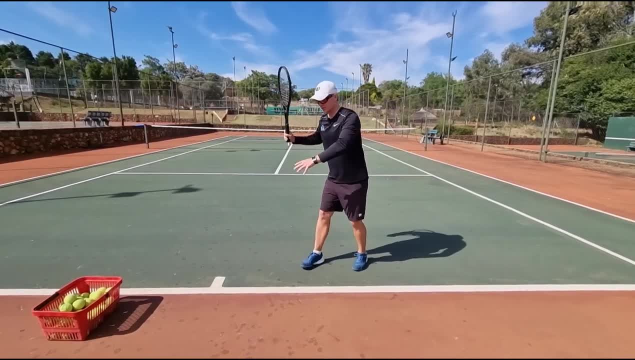 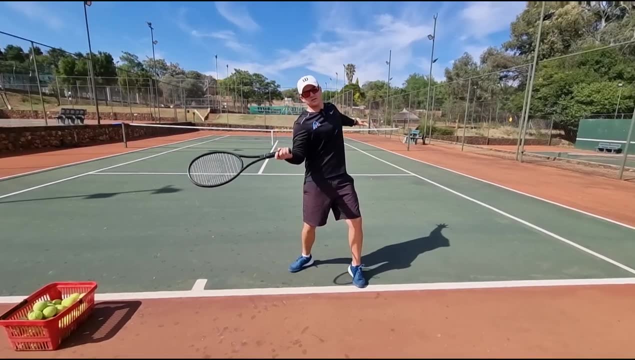 your left shoulder too soon. notice what the racket head does. So I'm in position if my left shoulder is pulling. look at the racket head. does it's facing up? Okay, I'm going to show you an example of what happens. if you hit the ball like that ball goes out. 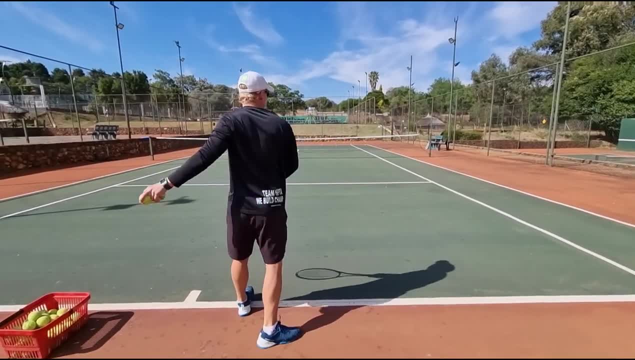 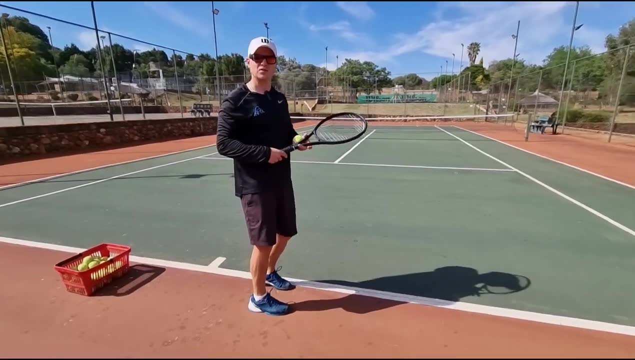 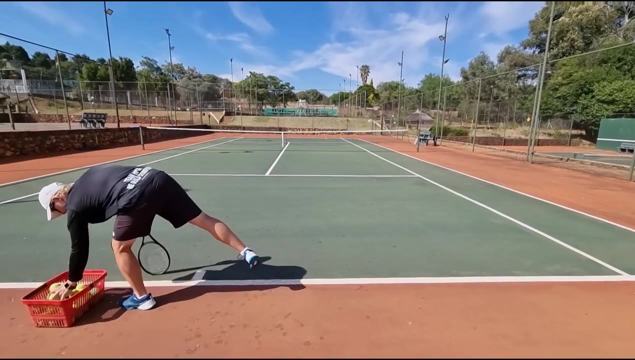 My left shoulder, I'm going to pull it. As I pull it, the ball just goes up. Go again. You could get lucky with timing, but again your consistency is going to be way out. I'll give you one more one: with my shoulder. pulling goes out. So what you want to do is again it. 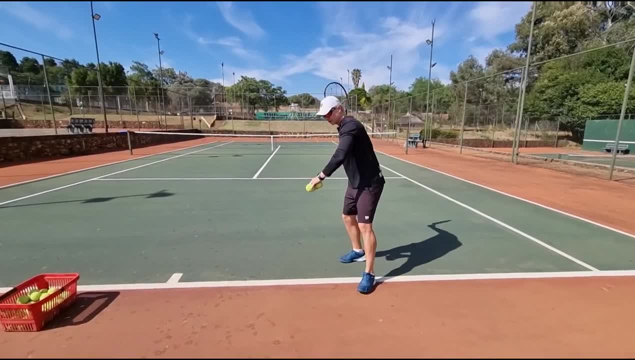 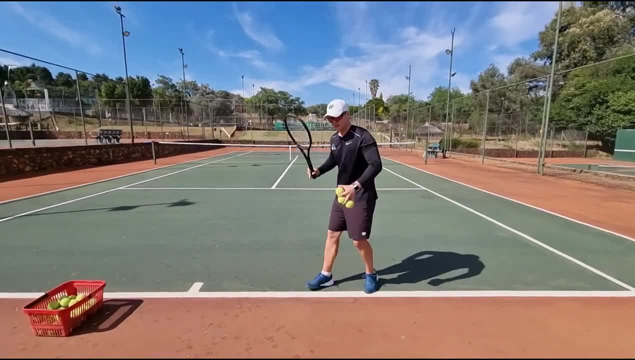 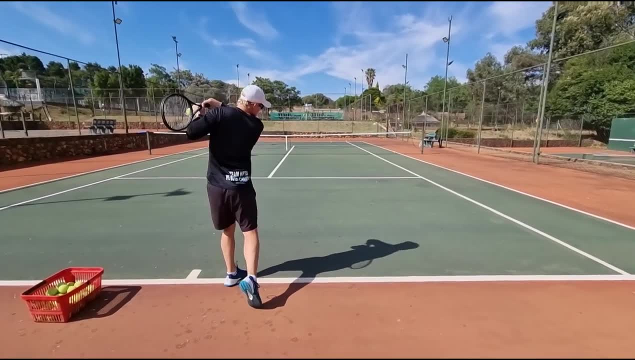 There's a reason why they keep their head on the same side. They keep their head still Because if you keep your head still, your shoulder cannot pull the ball out. Okay, so it should look like this, Still relaxed in my hand. 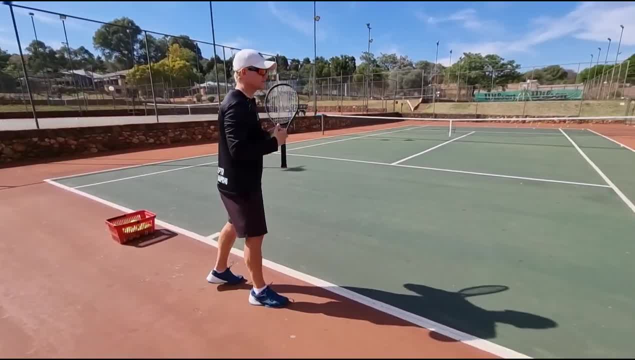 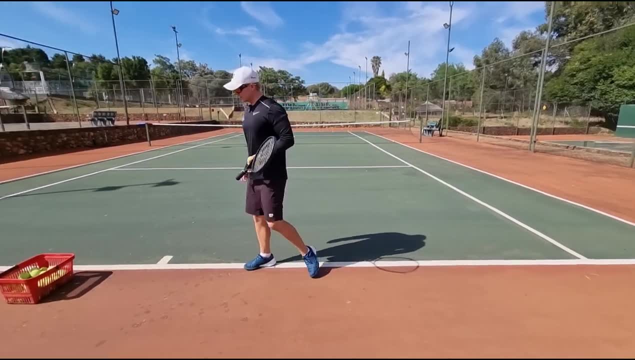 Boom. So, whatever you want to tell yourself, keep your head over the ball, keep your head still, keep your eyes watching the ball. That's going to help you not to pull your left shoulder. Okay, Okay. then last thing, guys, I can't not talk about this. 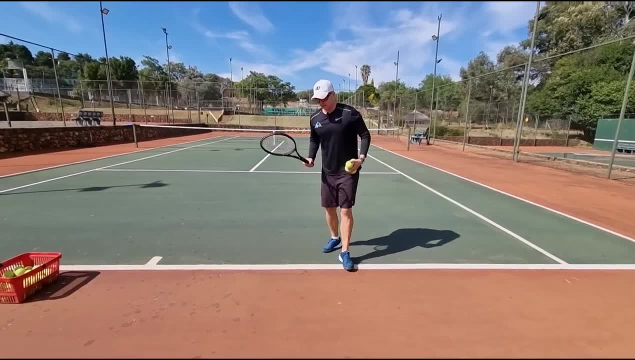 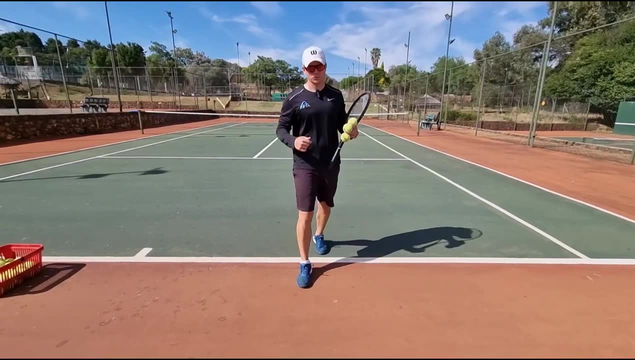 It's so important. it's the balance. Okay, once again, think about it. If I'm hitting the ball, and as I'm hitting it, I'm losing my balance backwards. It's a very common mistake. players fall back, they fall back. 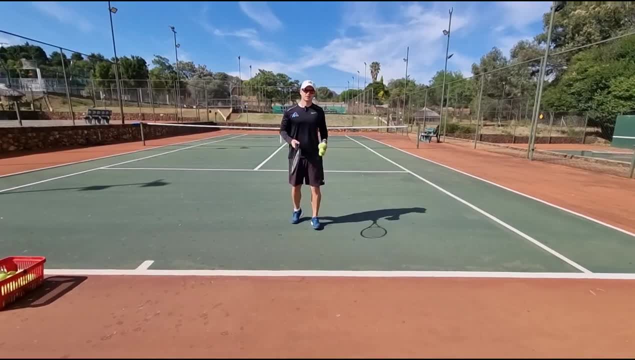 Once again, my racket head. as I fall back, my racket head is going to go up. Okay, it's going to look something like this. I want you to understand, though: there's all these tips, they work together. You can't do one without the other. 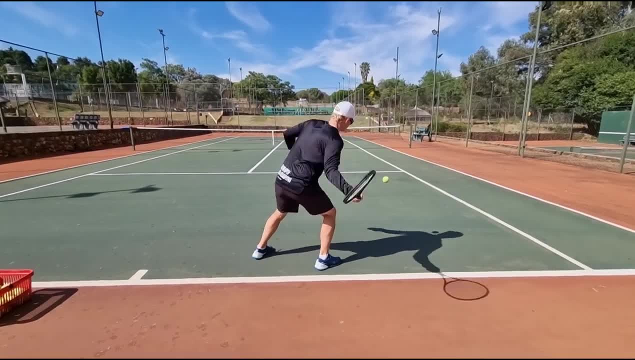 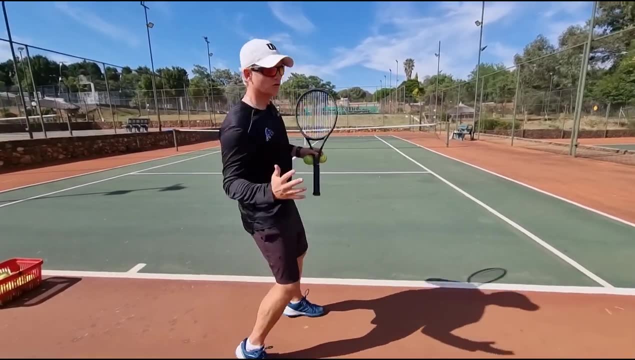 They're all linked together. So this is me in position, falling back- Very common mistake. especially when players are under pressure and the player is pushing them back, they fall back. Okay, What you want to do is you want to get into position? go back first. 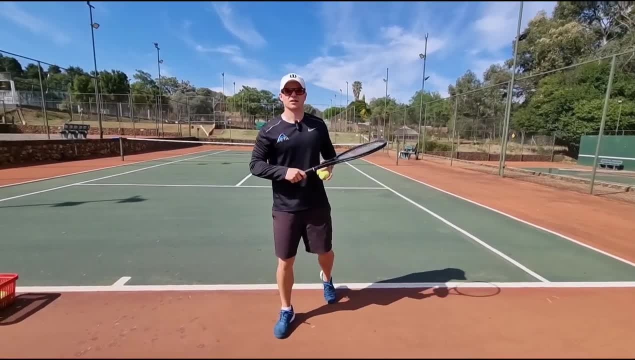 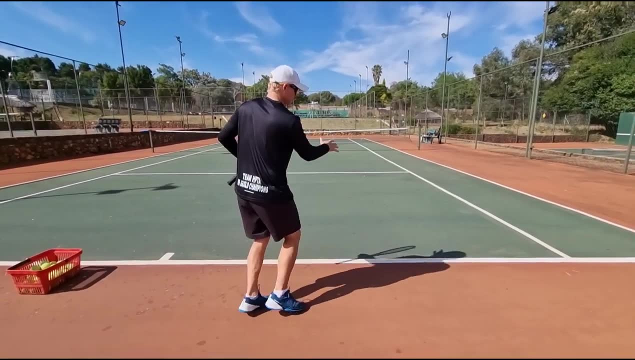 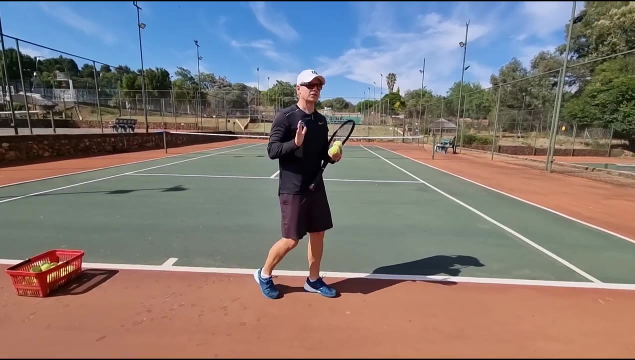 so you have enough time to still go forward. Okay, If the ball goes back and deep ball goes back and deep shuffle back, so you have enough time to go forward. So it should look like this: Just imagine your body weight is always going a little bit forward off the contact point.